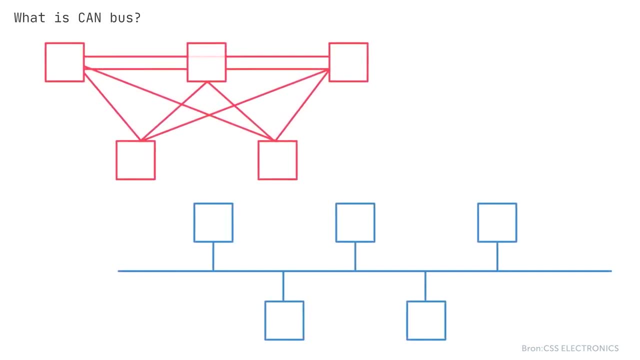 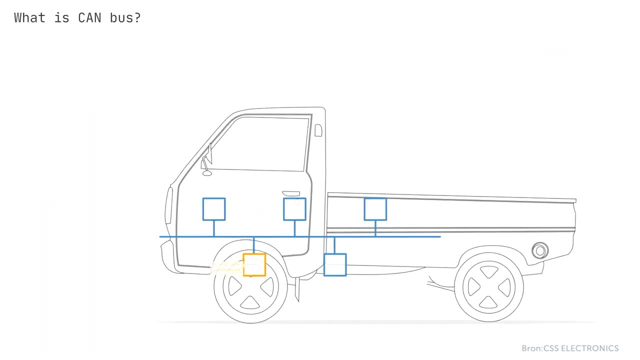 The CAN bus system enables each ECU to communicate with all other ECUs without complex dedicated wiring. Specifically, an ECU can prepare information, for example sensor data and other data. The CAN bus system can also manage the sensor data and broadcast this via the CAN bus. The 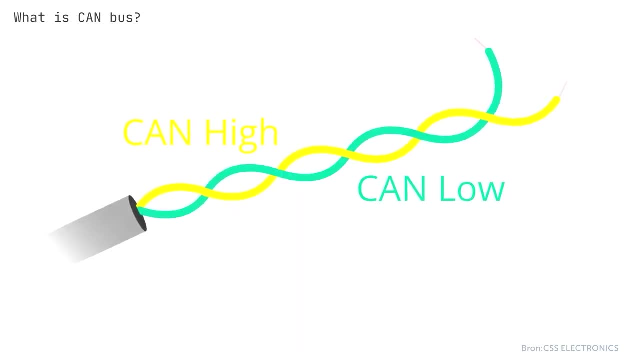 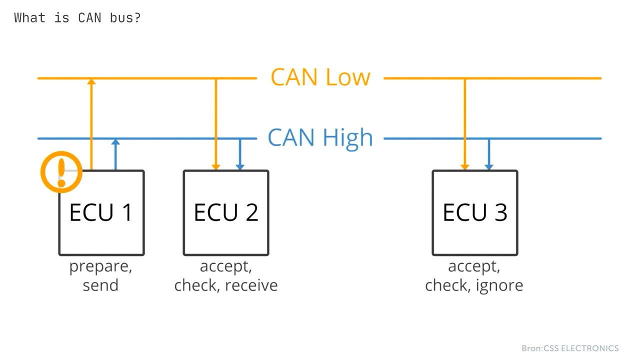 physical communication happens via the CAN bus wiring harness, consisting of two wires – CAN low and CAN high. The broadcasted data is accepted by all other ECUs on the CAN network, and each ECU can then check the data and decide whether to receive or ignore. 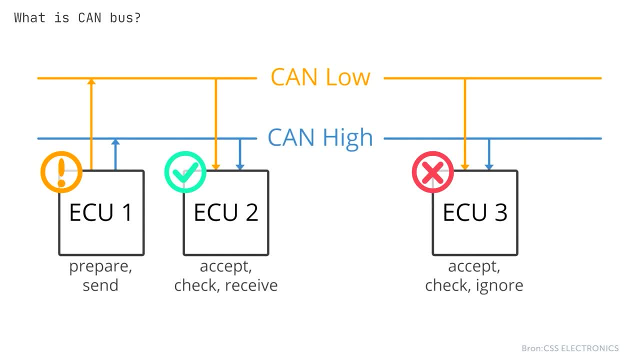 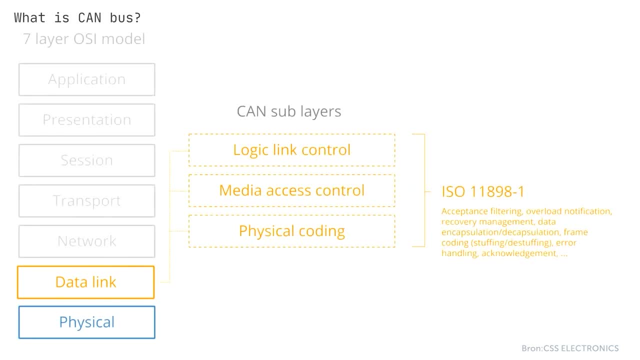 it. In more technical terms, the controller area network is described by a data link layer and physical layer. Specifically, ISO 11898-1 describes the data link layer, while ISO 11898-2 describes the physical layer. Today, CAN bus is standard in practically all. 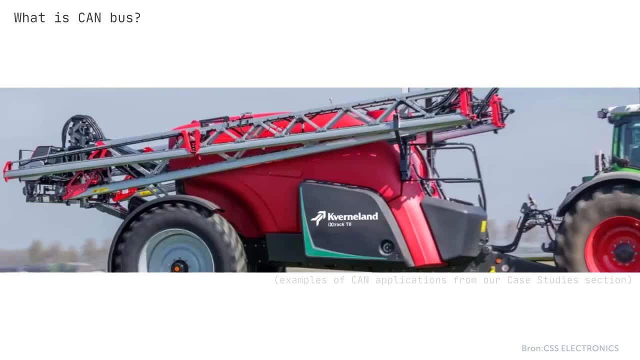 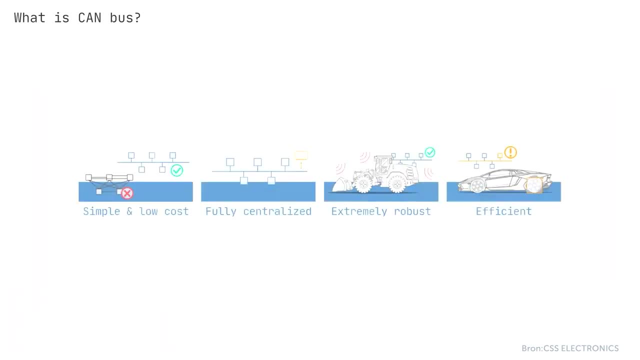 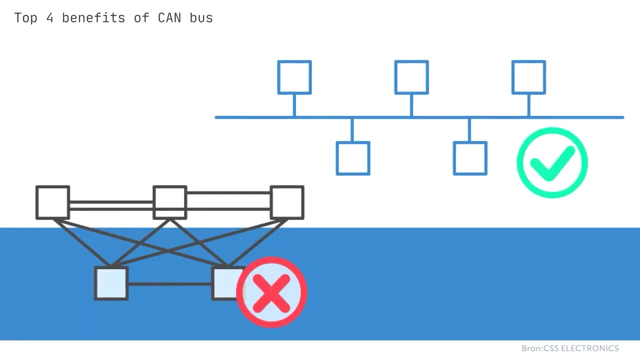 automotives like cars, trucks, buses, tractors, bikes, as well as ships, planes, EV, batteries, machinery and more. There are four key benefits to CAN bus that help explain the popularity. First, CAN bus is simple and low-cost. Easy use. communicate via a single CAN system instead of 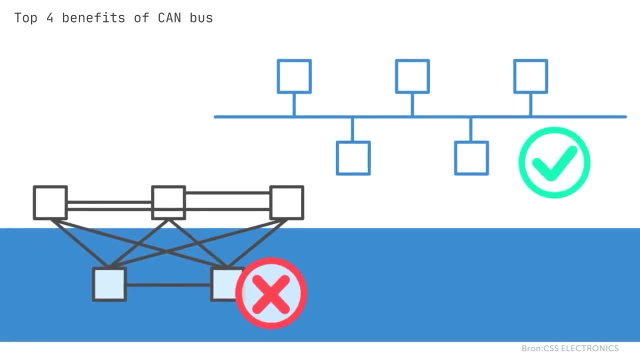 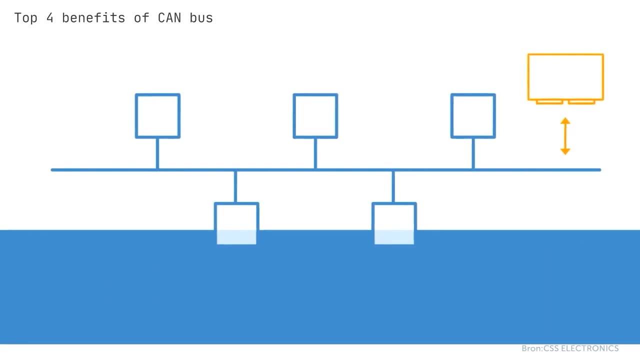 via direct, complex analog signal lines, reducing errors, weight, wiring and costs. Second, it is fully centralized. The CAN bus provides one point of entry to communicate with all automotives. The CAN bus provides one point of entry to all automotives. 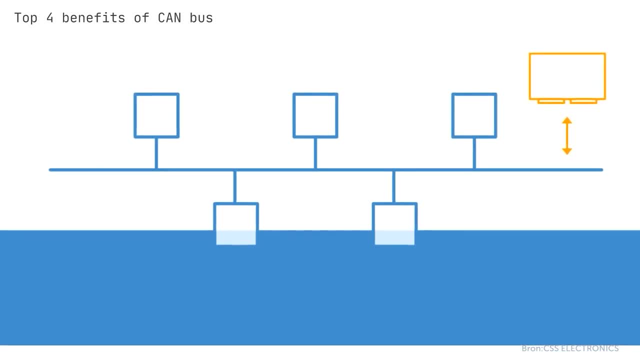 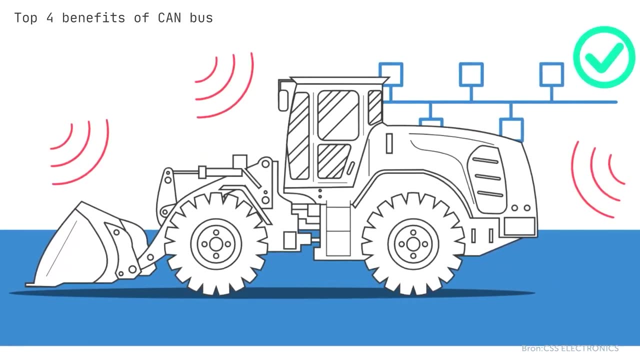 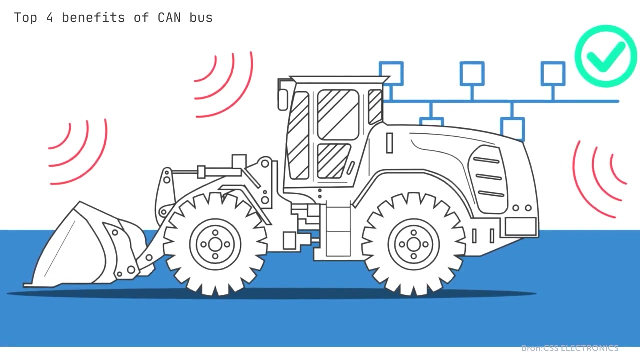 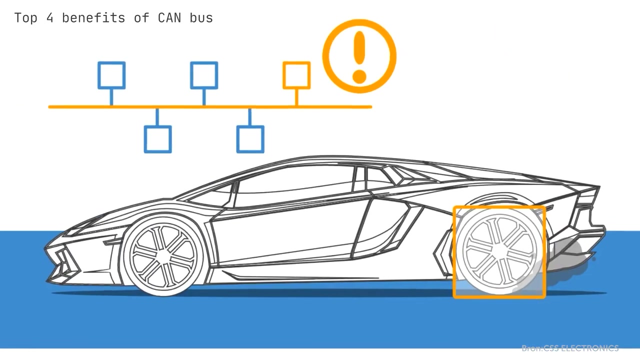 All network ECUs enabling central diagnostics, data logging and configuration. Third, CAN is extremely robust. In particular, the system is robust towards electric disturbances and electromagnetic interference, making it ideal for safety-critical applications. Finally, it is efficient. CAN frames are prioritized by ID, so the top priority data 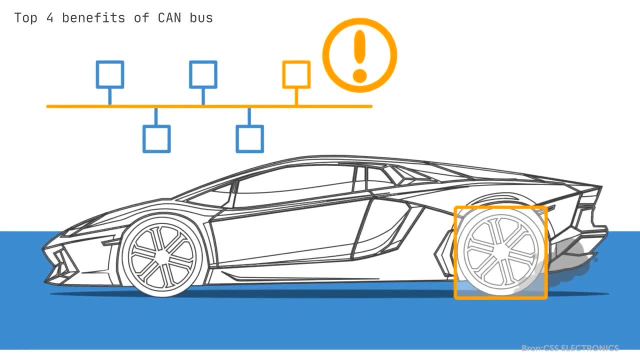 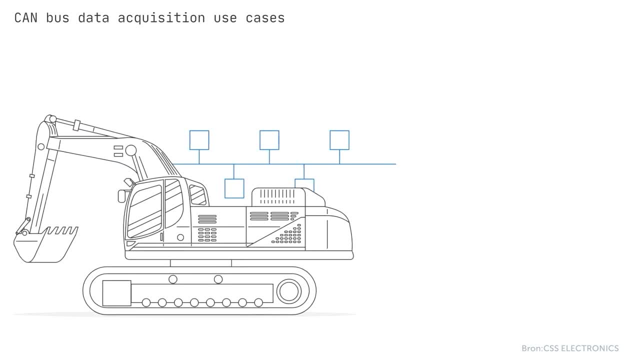 gets immediately to the system. The CAN bus is a very efficient system. It provides immediate bus access without causing interruption of other frames. Truly understand the CAN bus protocol. We find it useful to explain how to record and decode CAN bus data. CAN data acquisition is done across many use cases today.